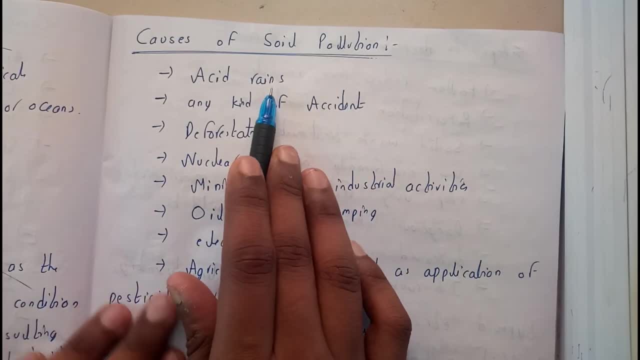 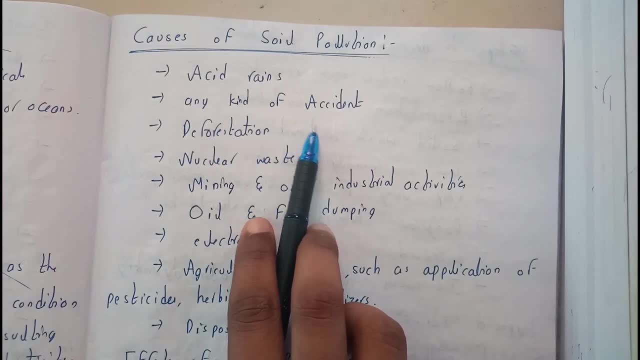 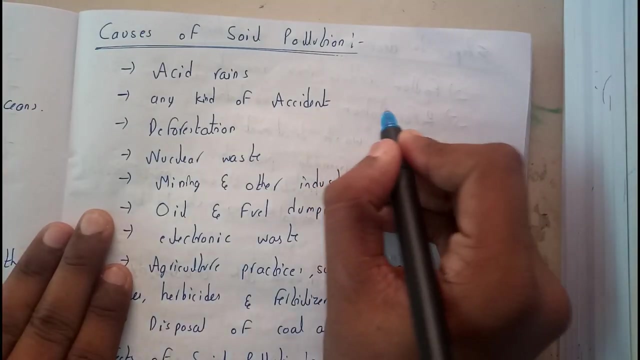 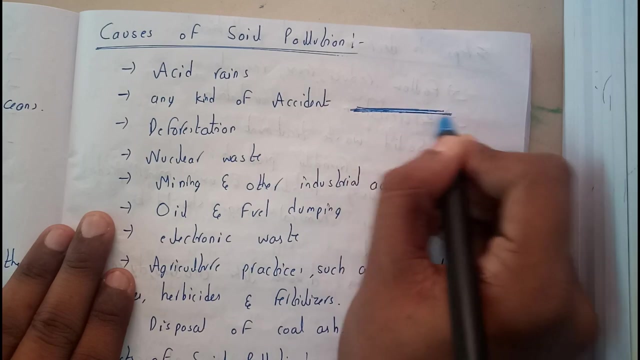 Acid rains. I told you about it. So acid rains even causes soil pollution, and any kind of accidents- Okay, even any kinds of accidents- even cause soil pollution. Yes, and deforestation, Everyone should know this, that the so everyone knows that the cultivation go, cultivation is done on soil, something like that. Okay. so 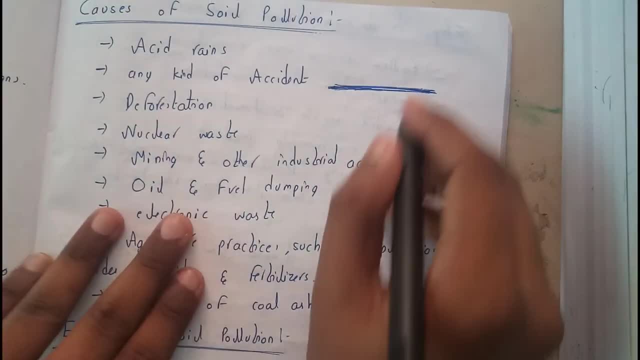 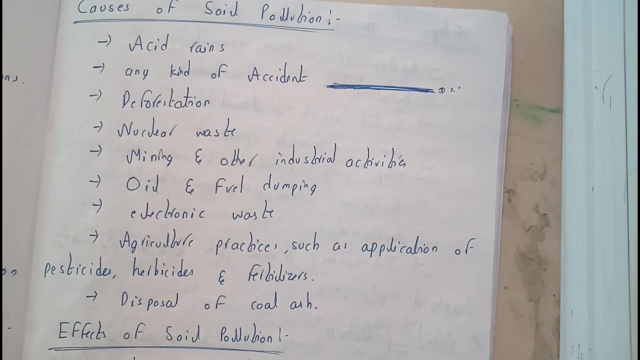 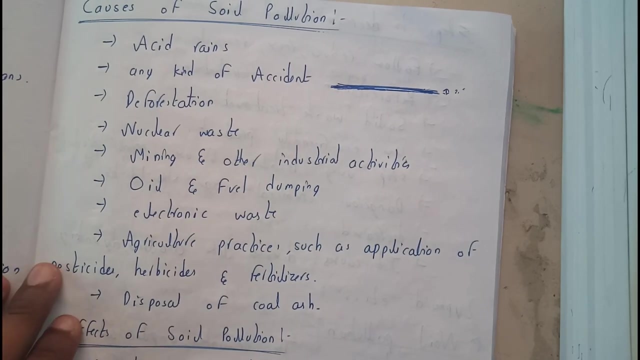 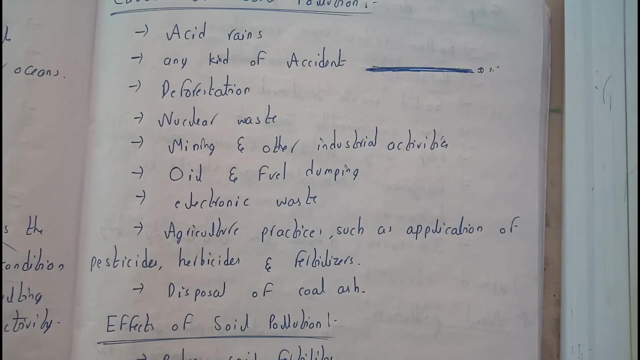 they and we'll be having some fertile land. We will be calling the fertility. So only 2.5 centimeters of the upper layer of the soil is the most fertile soil. The lower part is just soil. That's it. Only the upper part is the most fertile soil and whenever an accident or something happens there, it is going to just move off and there is no chance of growing crops properly. 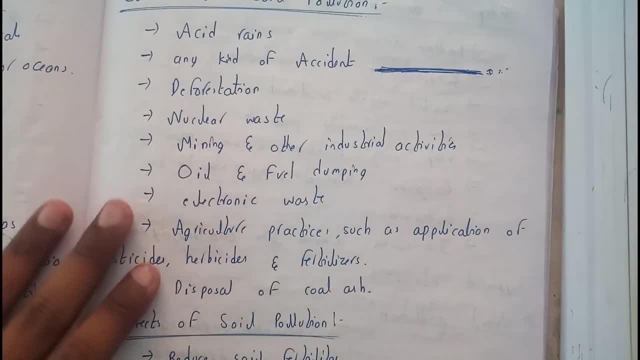 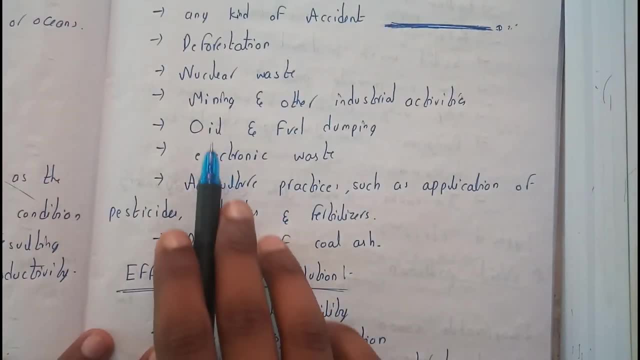 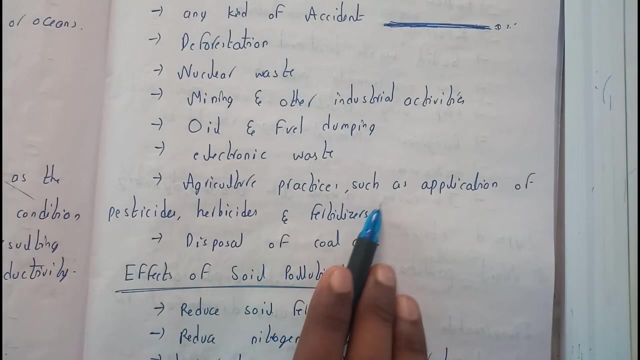 So causes of accidents also causes soil pollution, even deforestation, Throwing of nuclear wastes, mining and industries, industrial activities, oil and fuel dumping: Yes. electronic waste like batteries: Yes. agricultural practices such as application of pesticides, herbicides and fertilizers: the main reason. 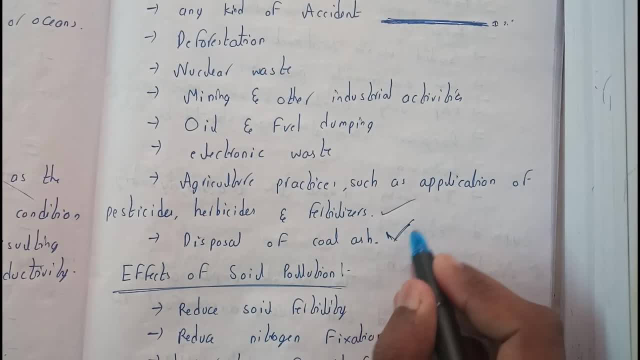 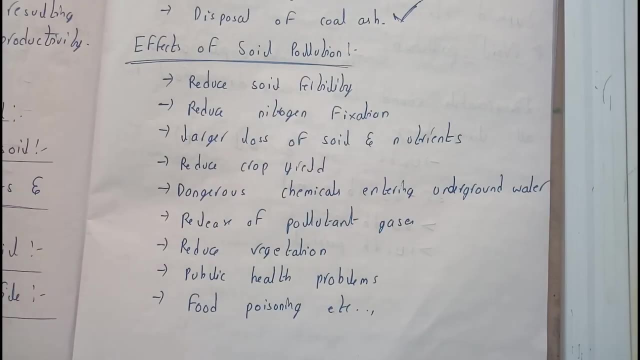 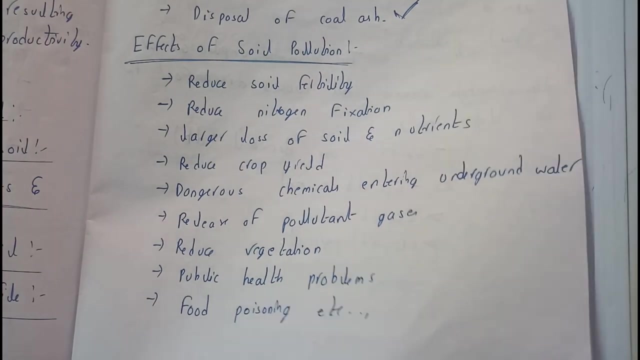 disposal of coal ash. I Hope everyone know about this coal ash. while generation of electricity Will be getting electricity from burning of coal, After burning the coal, the left out thing is just like a powder that is called as a coal ash. Okay, guys, I hope everyone is clear with effects- Sorry, causes- of soil pollution. So now let's go through effects of soil pollution. Okay, 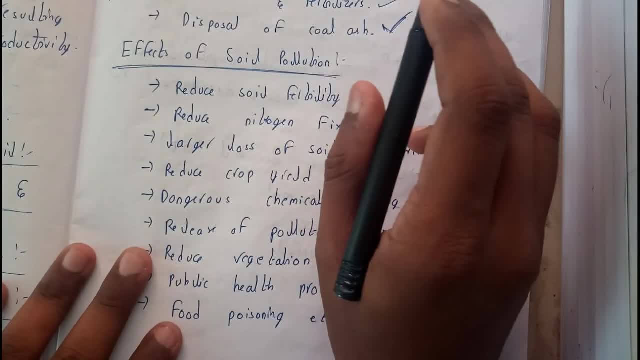 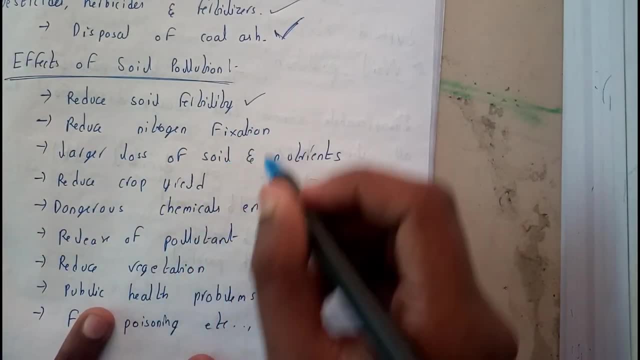 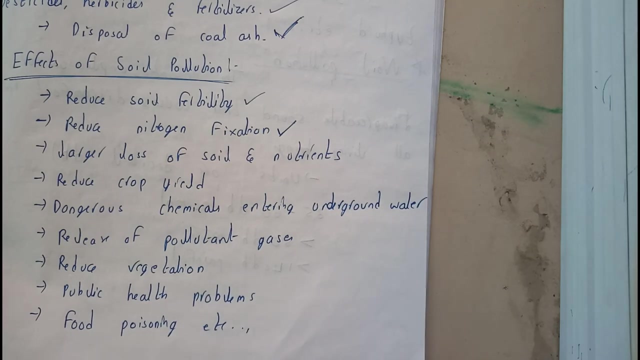 Soil pollution. it reduces soil fertility, which we have discussed above, which is 2.5 centimeters, the only fertile land. It reduces nitrogen fixing. So nitrogen fixing is a property that I hope everyone knows That in our surroundings will be having. at most, maximum percent is nitrogen and nitrogen is one of the most important. 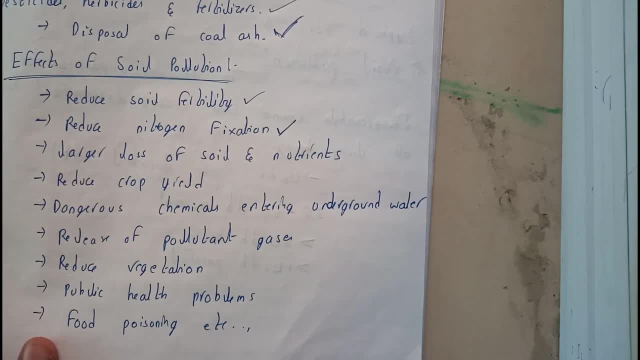 Protein or nutrient for plants. They'll be taking off nitrogen and they're believing of nitrogen and it's a huge cycle. guys, We'll be discussing in one chapter, in some chapter, I hope I remember, in second chapter Maybe we'll be discussing about this. Don't worry, guys, be cool, We're gonna go through it. So it reduces nitrogen fixation and large loss of soil and nutrients. Yes, soil pollution causes loss of soil fertility, which leads to loss of soil. reduces crop yield. Yes, we have discussed it. next, dangerous chemical entering underground water.